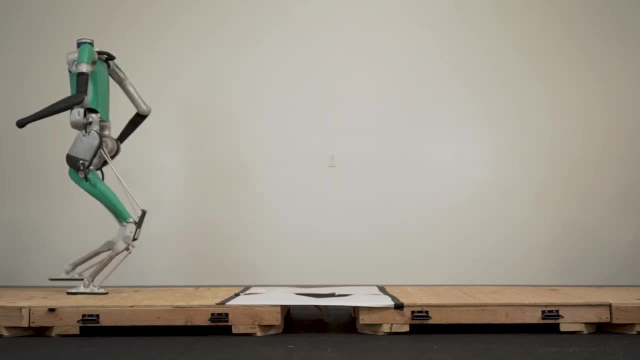 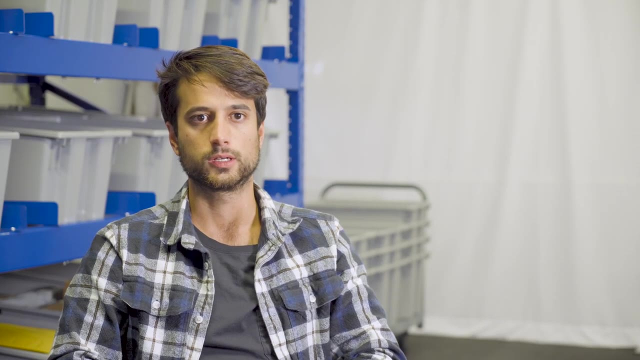 structure of an animal. but just trying to copy the performance of an animal, we end up with really similar behavior that has sort of these animal-like characteristics. In order to really understand this phenomenon, we can go to a laboratory setting. So here we have a guinea fowl. that was basically. 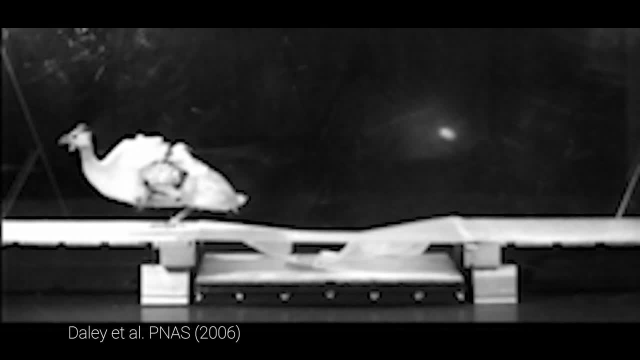 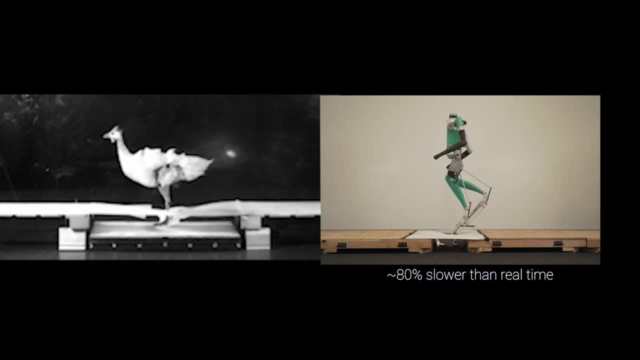 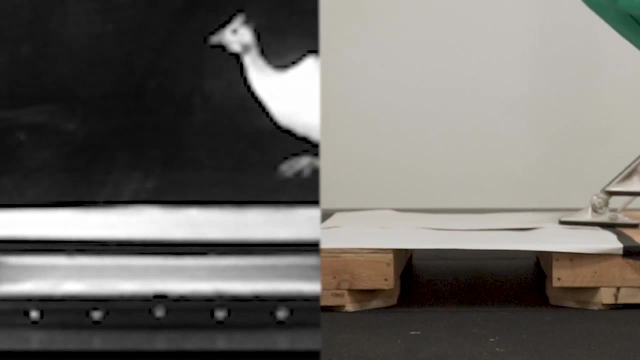 running down a corridor and there's this hidden hole in the ground that the experimenters have hidden from the bird. Similarly, we kind of set up the same situation for Digit and here we can see side by side how they respond to that similar disturbance. So, as you can see, in both cases 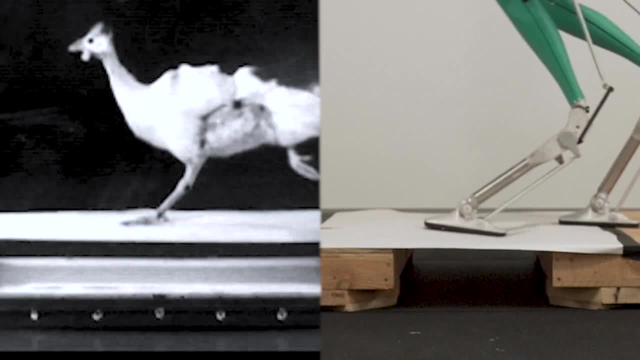 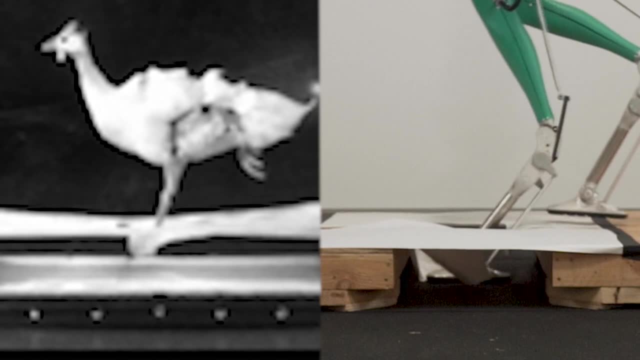 first the foot slows down, kind of anticipating hitting the ground, and that foot starts to apply forces on the ground or tries to, But obviously, since there's tissue paper there, it just bursts through the tissue paper and accelerates that foot straight towards the actual ground. 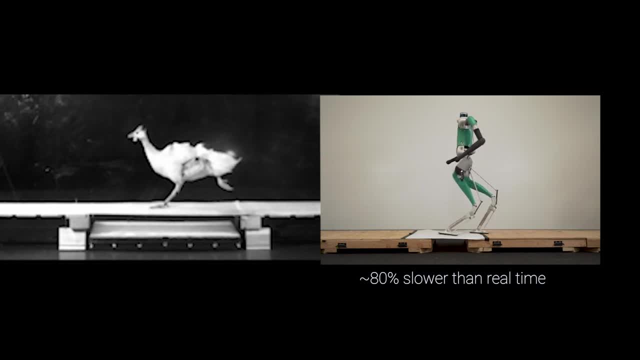 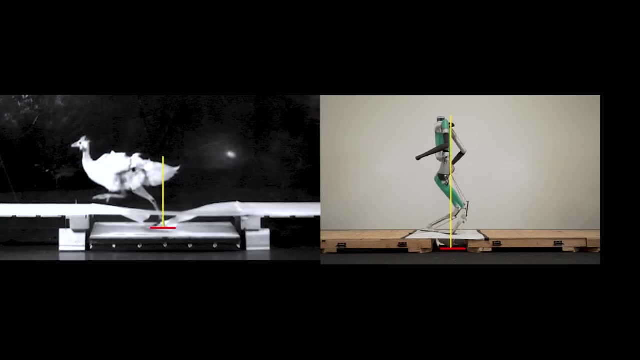 Because of that unanticipated disturbance, the foot swings back a bit further than the robot and the bird expects and you can see that it touches the floor at a point a little bit further back relative to the body than it was planning to, Because it's a little bit further back that. 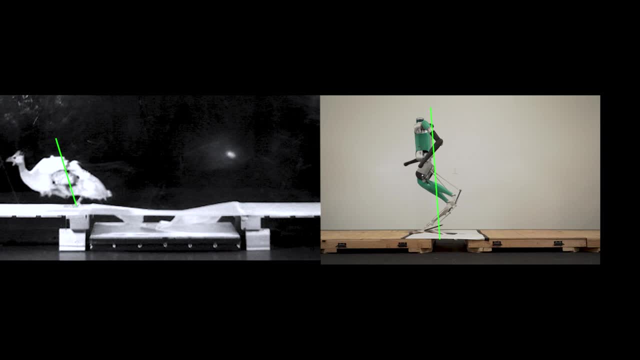 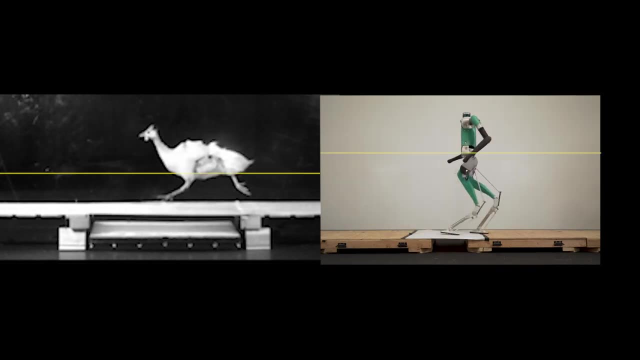 actually pushes the body forward and accelerates the body of both the guinea fowl and the robot forward faster than it expected. Now that the body is moving a little bit faster than it expected, that next step up is like an additional disturbance And both the bird and the robot have slightly more crouch postures. It does take a few. 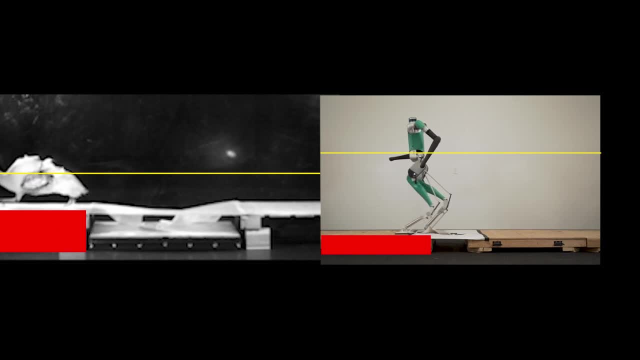 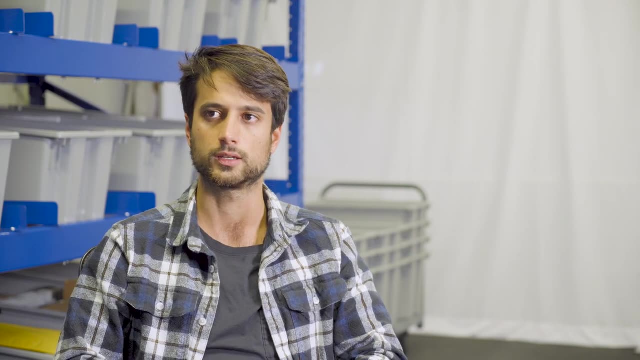 strides after this to slow down again to its nominal speed and also get the body back up to its original height relative to the ground. But what's really important to think about is, through all this, it had to do this in a fraction of the second. It had no idea that that disturbance was. 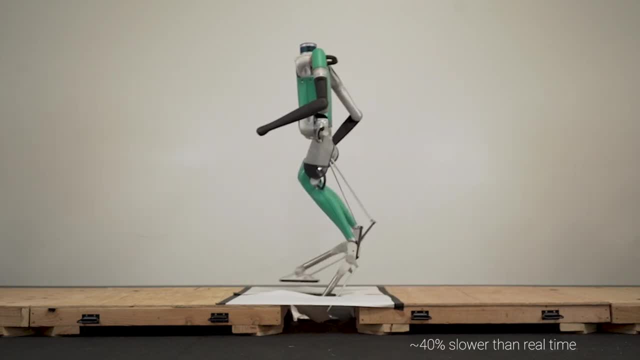 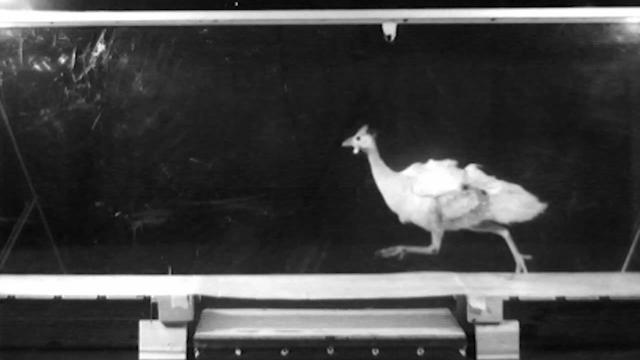 there It had to feel that disturbance with its foot and just reflectually deal with it in a really fast timescale. In the guinea fowl's case, it has generations and generations of evolution that have led it to have this kind of compliant, flexible structure to its leg and